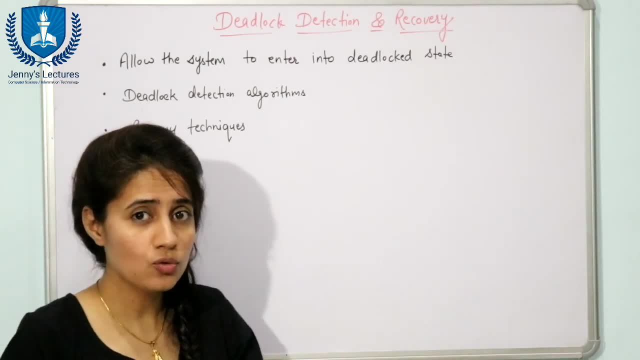 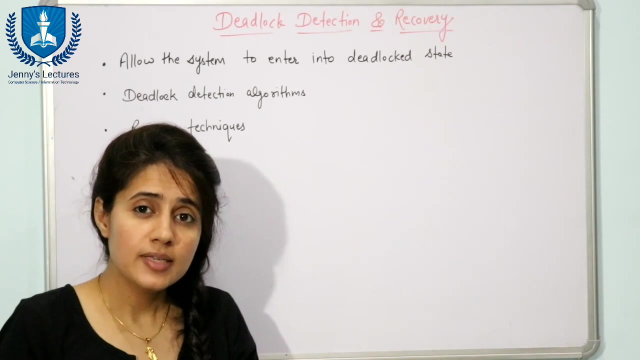 into deadlocked state. And once the system entered into deadlocked state, after that some deadlock detection algorithms would be applied. These are the algorithms which basically examine the state of the system at that particular point of time and then determines whether deadlock has arrived or not. And if yes, if deadlock situation is there, then finally, 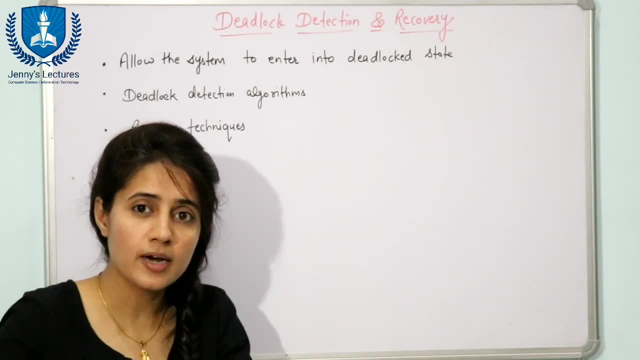 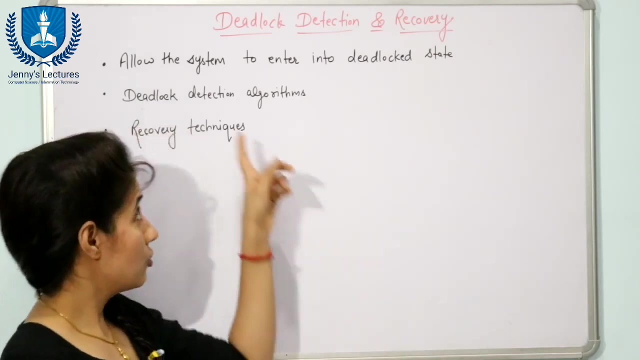 some recovery techniques would be applied to recover from that And if no deadlock is there, then finally, after some amount of time, again deadlock detection algorithm would be applied to determine deadlock has arrived or not. So in this video we are going to discuss only the deadlock detection algorithms and in next video we 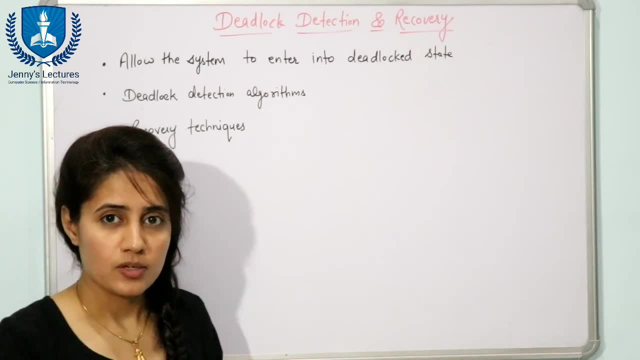 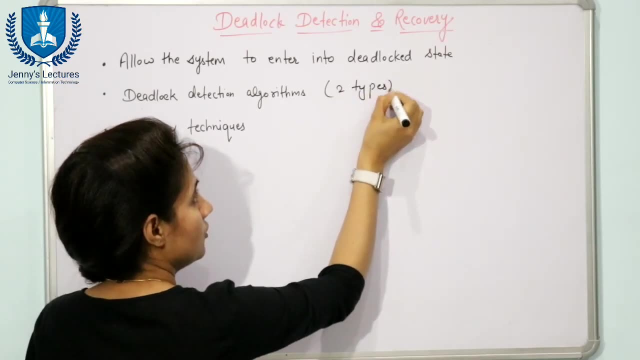 will discuss. what are the recovery techniques? Now, see, two types of deadlock detection algorithms are there. See, we have discussed in previous videos that resource allocation grammar and resource allocation grammar, And in this video we have discussed the resource allocation grammar. And in this video we have discussed the resource allocation grammar. 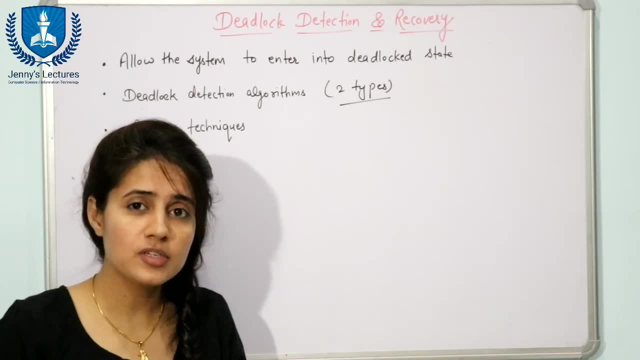 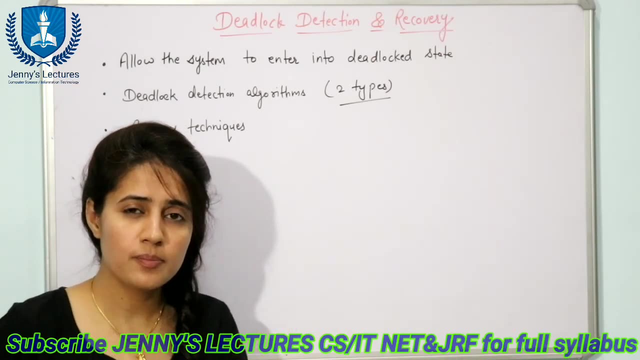 In that case, we have discussed resources are having single instance as well as multiple instance. What do you mean by multiple instance? As you know that if we have two CPUs in our system, then you can say two instances of CPU are there. If one CPU is there, then you 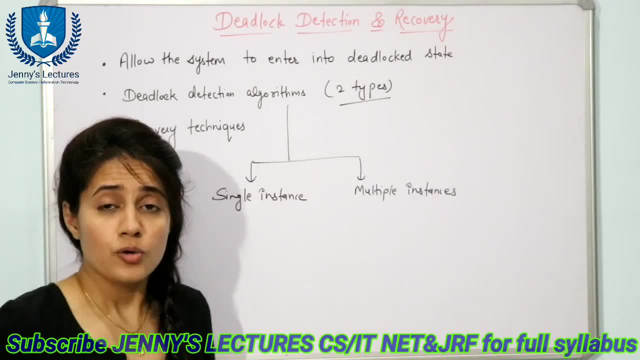 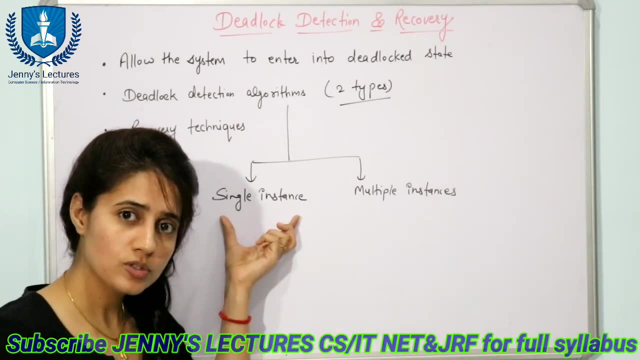 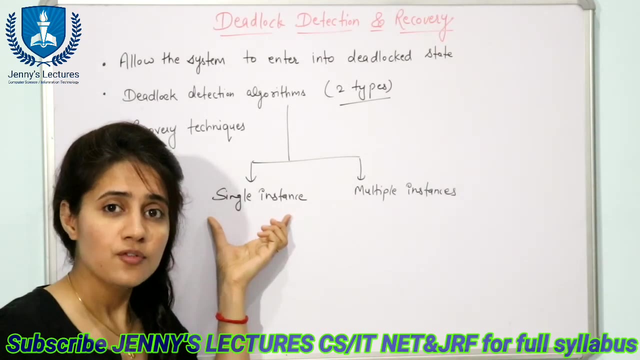 can say: single instance of CPU is there, Fine. So here two situations are there: That system is having single instance of all the resources and system is having multiple instances of. if single instance of resource is there, then which algorithm is used for detection the deadlock that? 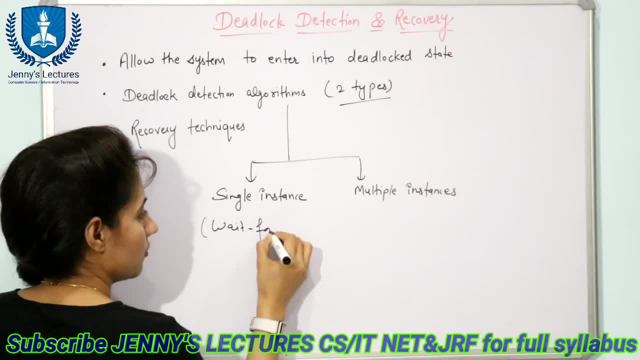 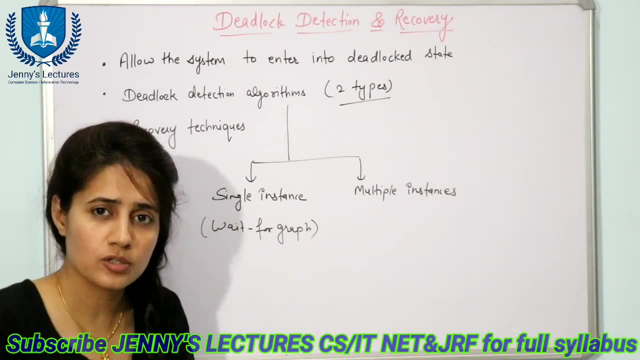 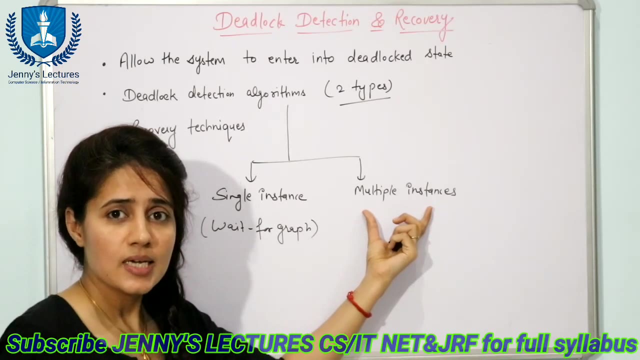 that is known as wait for graph. or you can say resource allocation graph. see, this wait for graph has enhanced version of that resource allocation graph. or you can say it's a variant of resource allocation graph. fine, and if multiple instances are there, then which algorithm is used then? 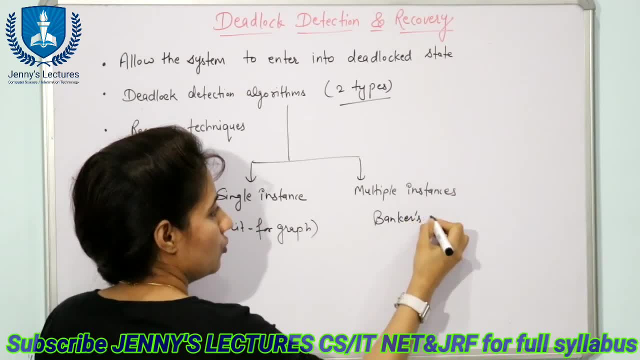 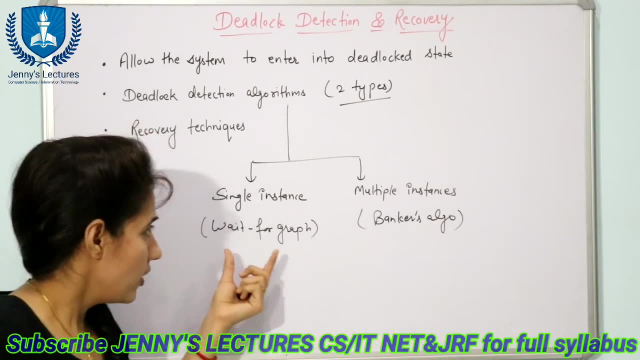 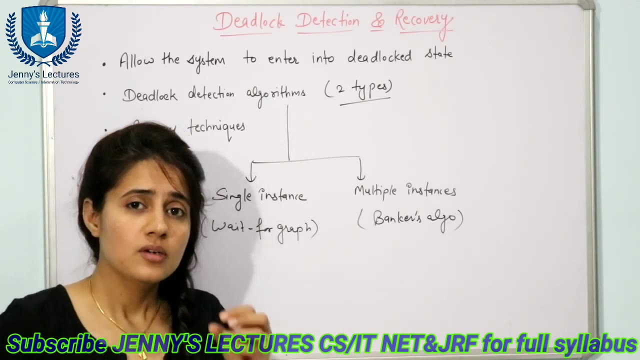 bankers algorithm would be used to detect deadlock, or you can say, a variant of bankers algorithm would be used. now, what is the difference between this wait for graph and resource allocation graph? see in resource allocation graph. as we know, graph is there, then obviously set of vertices and 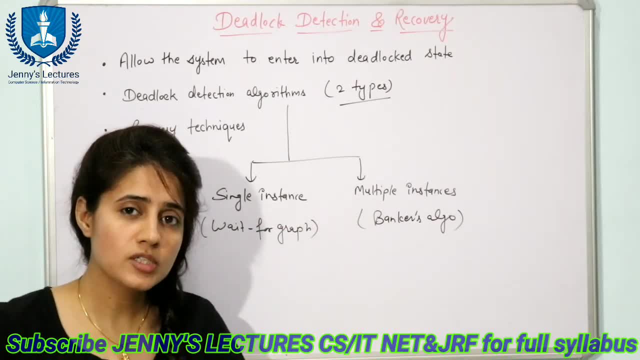 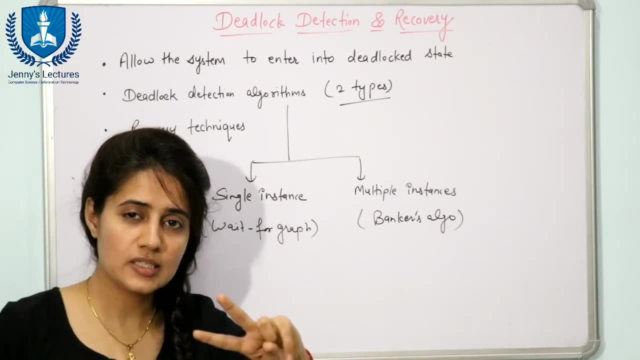 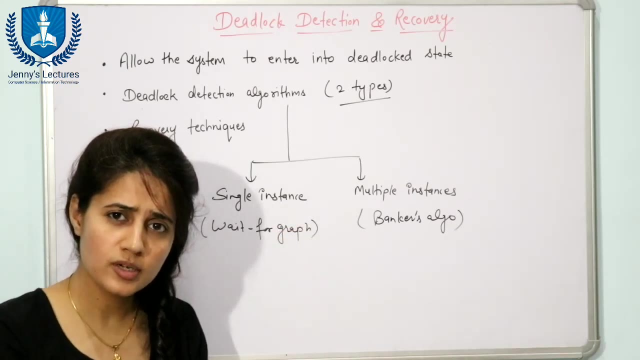 set of edges would be there and set of vertices. and resource allocation graph is what? set of processes and set of resources. two types of vertices are there, but we remove set, we remove resources from the resource allocation graph and then finally it becomes what wait for graph, or you can say that in wait for graph. 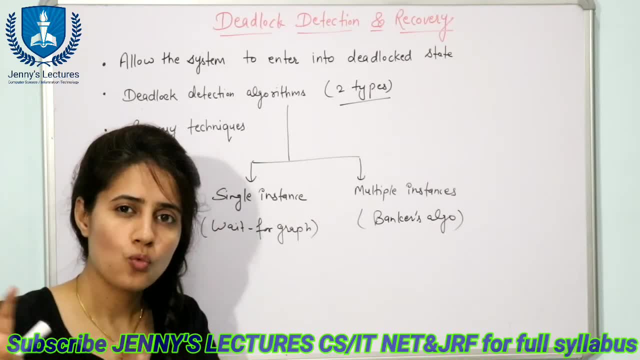 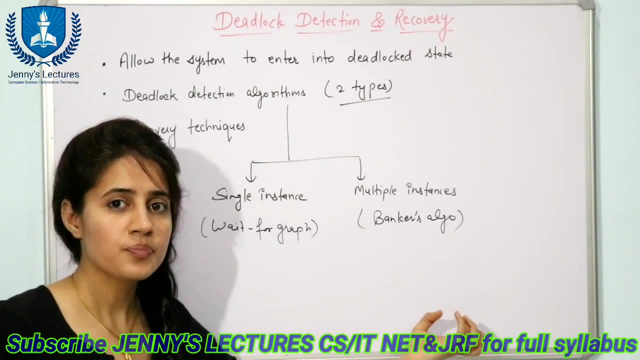 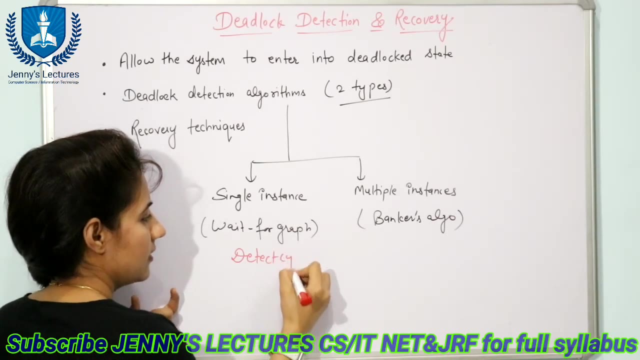 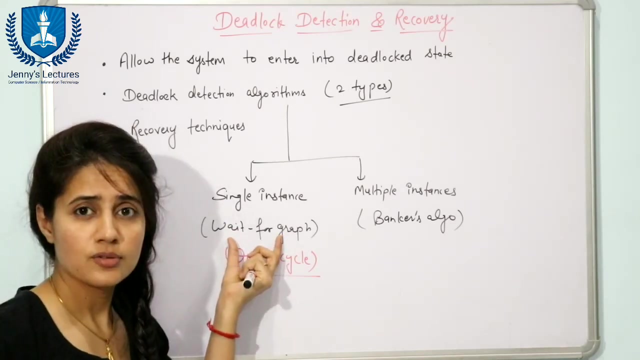 we have only processes as vertices in this graph. we'll discuss how a resource allocation graph will be converted into a wait for graph. so simple: funda is in wait for graph. we have just detect cycle. if cycle is there in wait for graph, then you can say that system is. 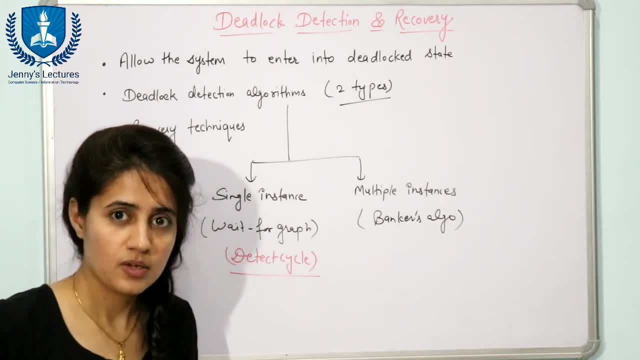 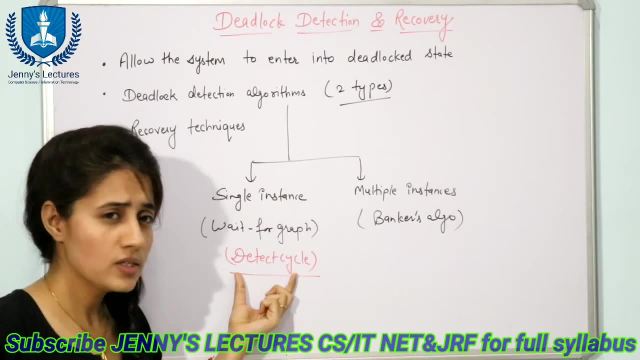 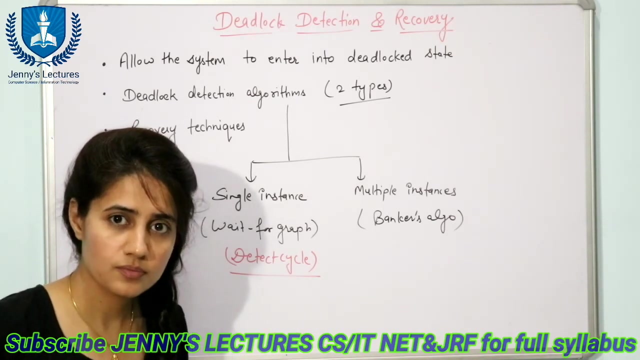 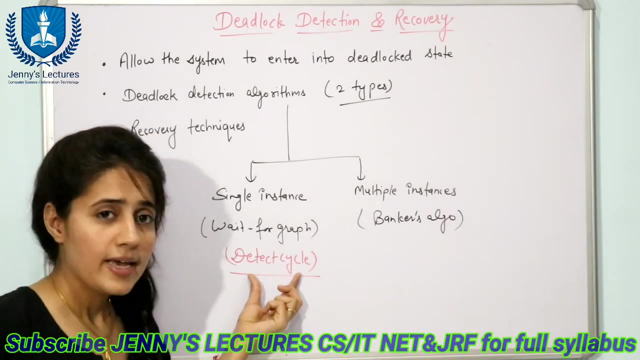 in deadlocked state? definitely in deadlocked state. so single instance of resources are there then the? this existence of the cycle in wait for graph is necessary and sufficient condition for deadlock, fine. but if multiple instances are there, multiple instances of resources, are there then existence of cycle in wait for graph? or you can say, in resource allocation, graph is only necessary. 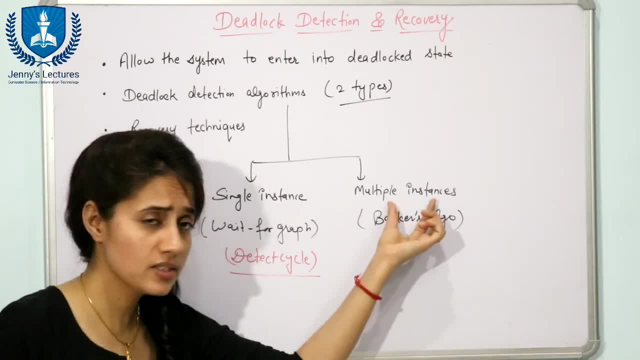 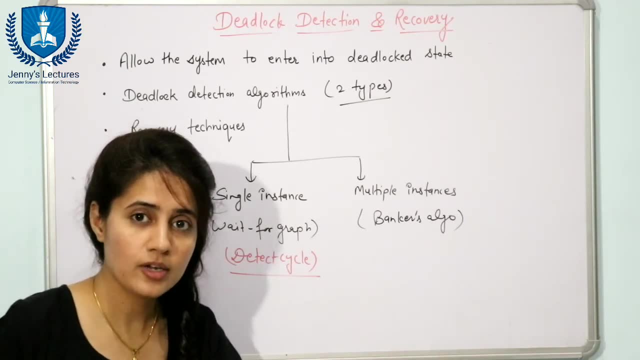 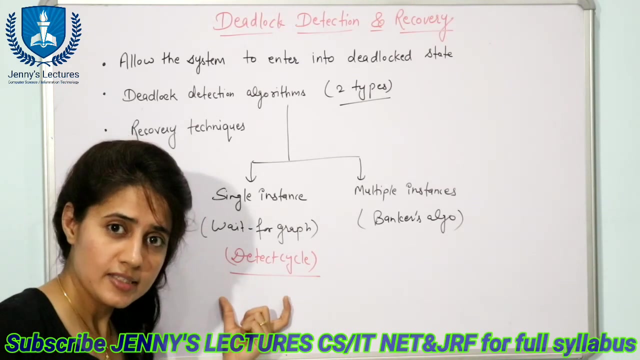 condition, not sufficient condition. if multiple instances are there and there is a cycle in wait for graph, then deadlock may or may not occur. we cannot say that if cycle is there, then definitely deadlock would be there, but if single instances of resources are there, then definitely deadlock would be there. 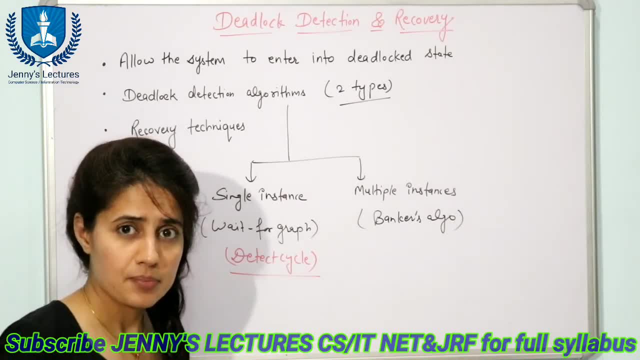 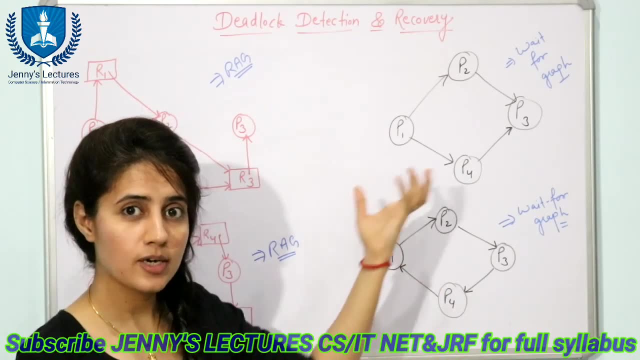 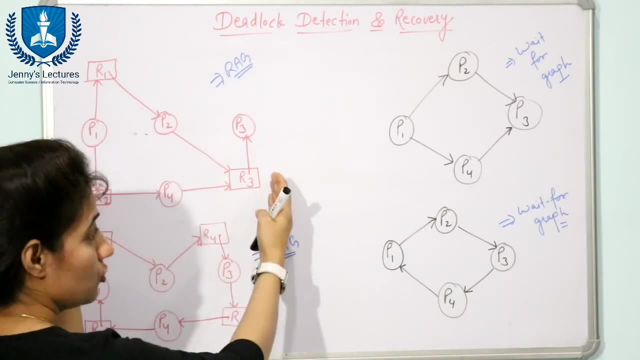 so we'll discuss both these techniques with the help of one example. so now, here we have two examples. one is this one and one is this one. one contains cycles means deadlock would be there, and another example does not contain any cycle- it means deadlock would not be there. fine, this is resource allocation graph and this is wait for graph. 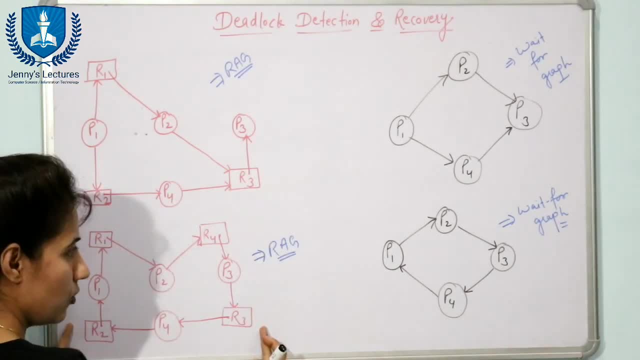 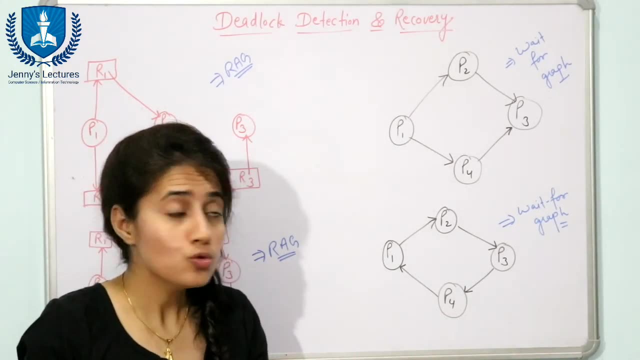 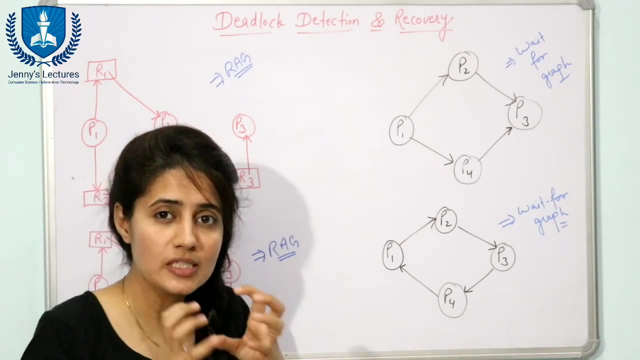 corresponding to this resource allocation graph. and this is another resource allocation graph graph for this resource allocation graph: fine, now see, system needs to maintain this wait for graph. fine, and then, periodically, an algorithm would be called on this wait for graph and that algorithm will do what that algorithm will: will search for a cycle in this wait for. 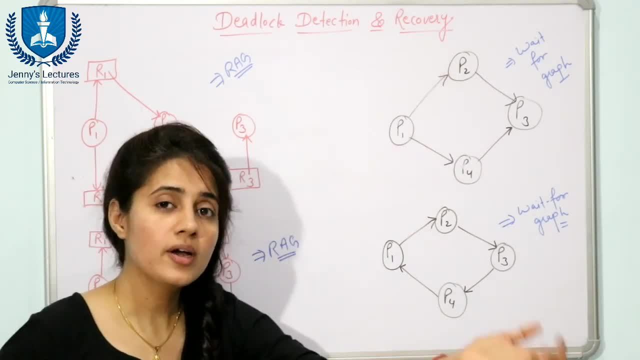 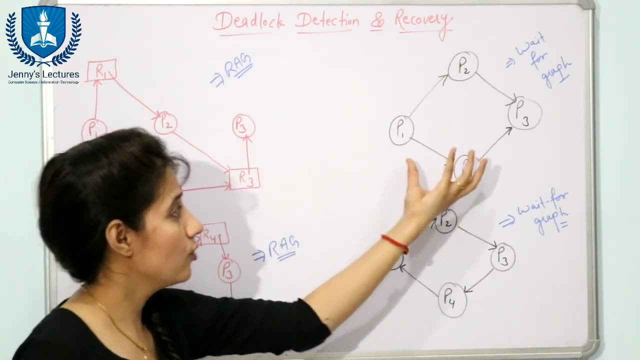 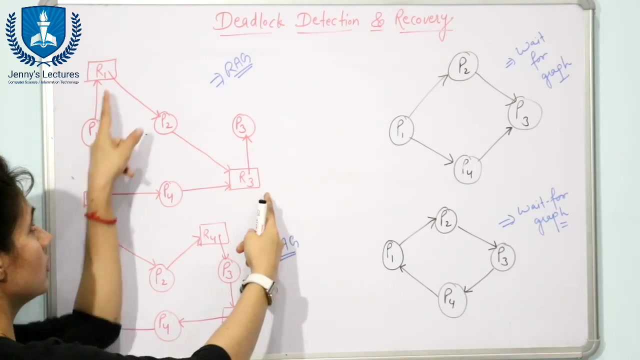 graph. and if cycle exists, then there would be deadlock, and if cycle does not exist, then there would be no luxury. fine, now how this weight for graph would be constructed from this resource allocation graph. see, it is in the resource allocation graph. we are, we are having processes. 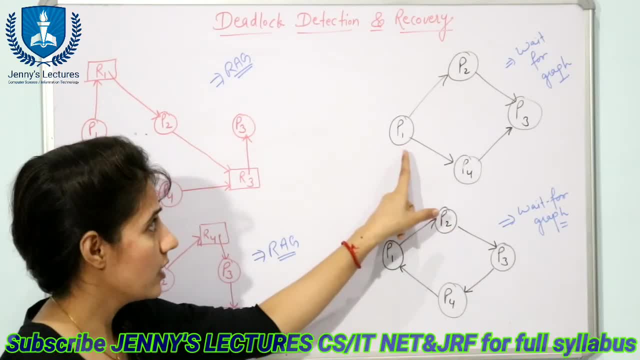 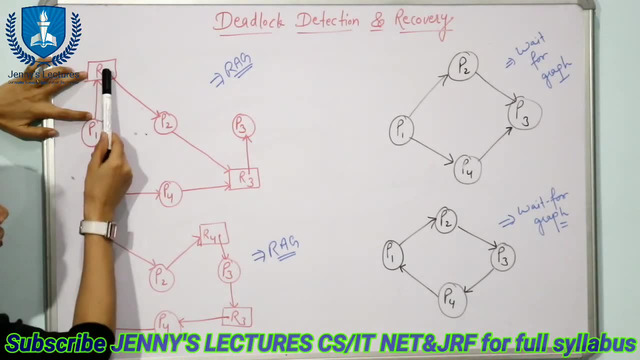 plus resources, but in weight for graph we are just having processes. see this kind of thing. this edge is from p 1 to r 1, means p 1 is waiting for r 1, but this r 1 is held by which process, p 2. so 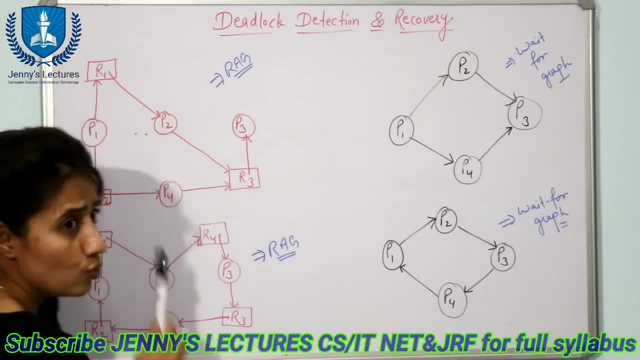 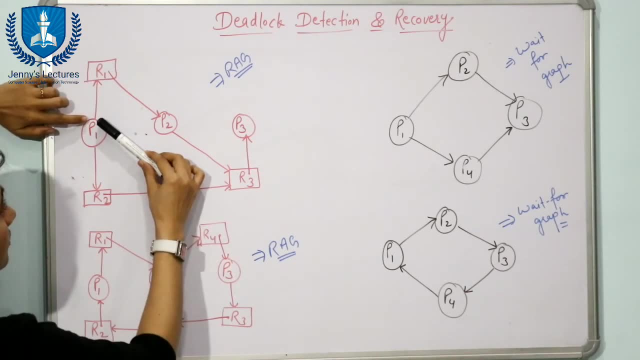 ultimately, scene is what p 1 is for, p 1 is for r 1, p 2 is going to postpone process, cross process, then this end stays for f, normal transition r- and rather the rest space is for f is waiting for p2 to release r1. fine, so simply, we remove this r1 and we simply just, you know. 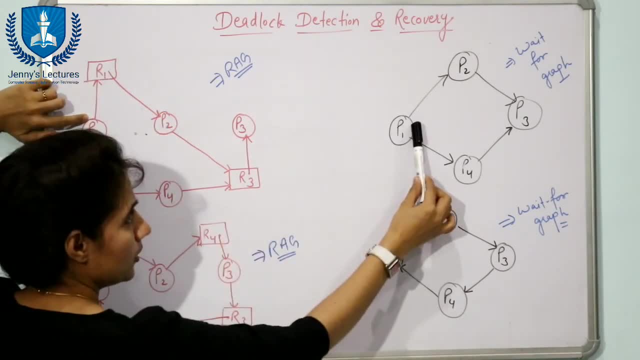 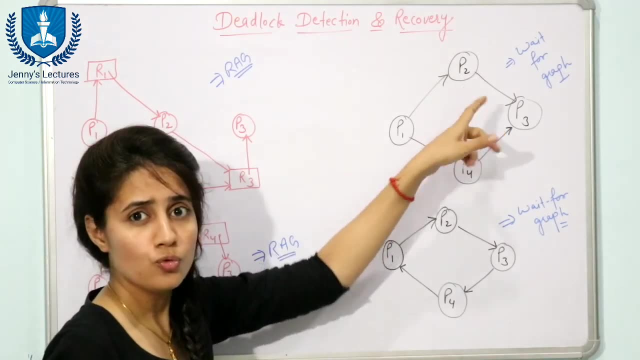 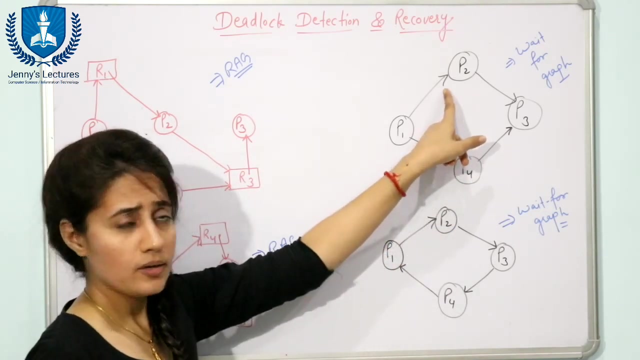 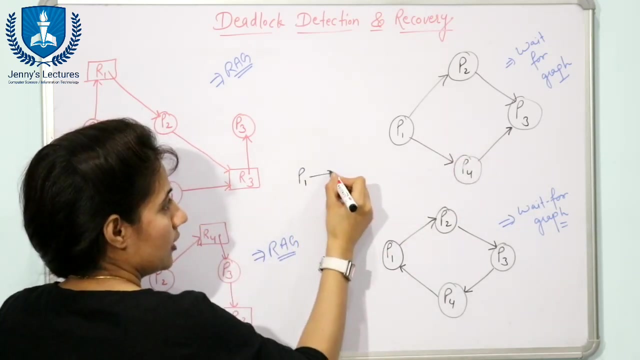 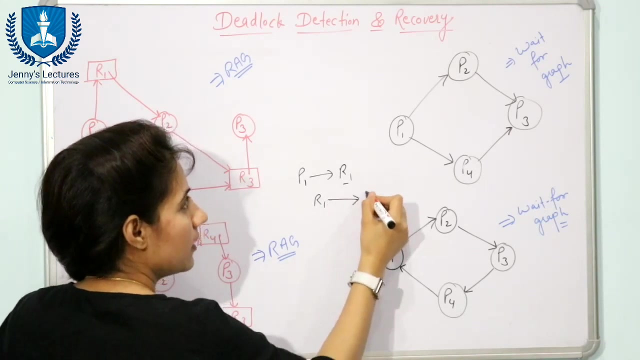 do this edge from this to this, so finally from p1 to p2. it means see, this edge means p1 is waiting for p2 to release a resource, fine, and this edge, something like that, would be in there in wait for graph if, if p1 is waiting for some resource, suppose r1- and this r1 is held by p2, if this 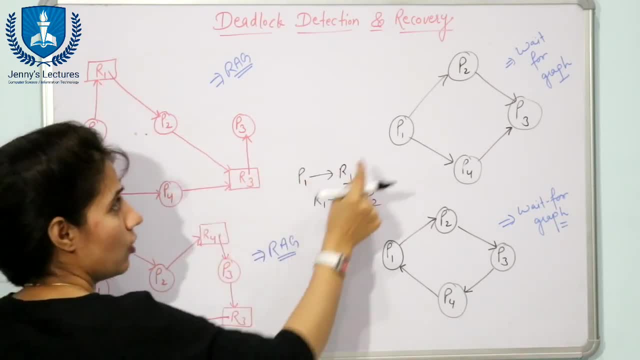 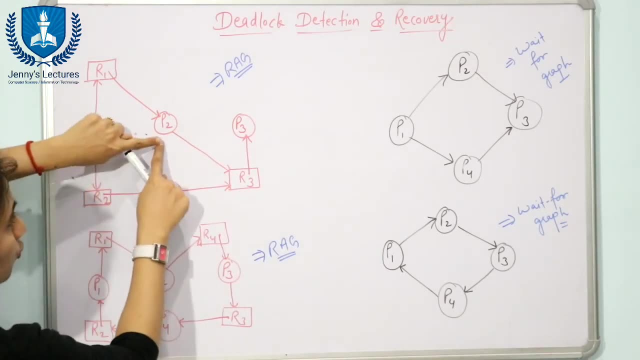 kind of scene is there in resource allocation graph. then only edge would be there from p1 to p2. so same same with p2, see p2. p2 is waiting for this r3. but this is an inch from the initial went position torition. so this in this means p2 is waiting. 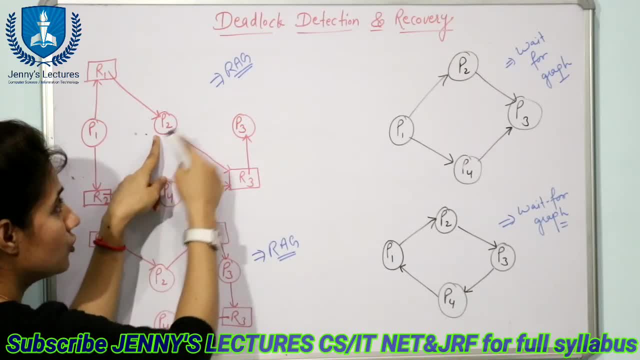 for p2 to release possible end. so now this is a little bit at isso curve. so just simple: % to$ of p1. so just for your map i can write down some untuk to% potatoes, super, i cannot. r3 is held by p3, so ultimately p2 is waiting for p3 to release this r3, right? so so there would be. 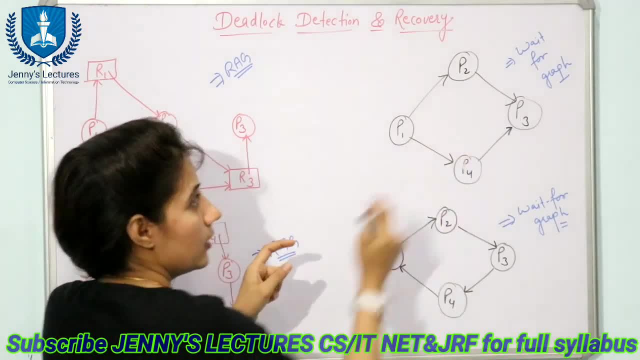 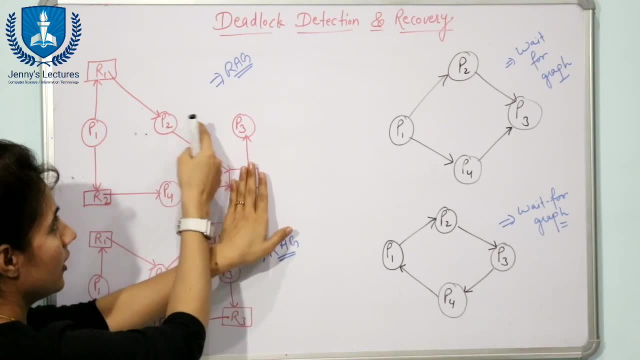 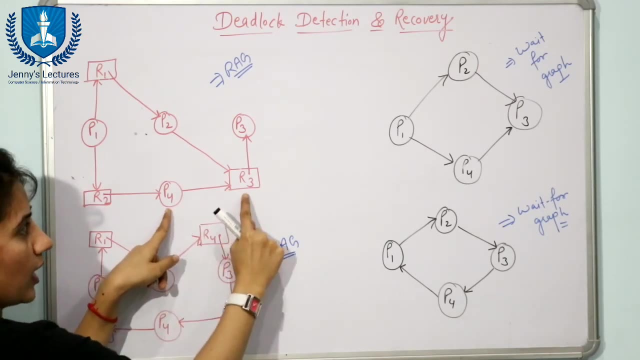 an edge from p2 to p3. see from p2 to p3. just remove this resource and see this arrow. is this? this arrow is like this, so just simply put an arrow from this to this same. with this, you can say: with p4, p4 is waiting for r3, but r3 is held by p3. so you can say: p4 is waiting for p3 to 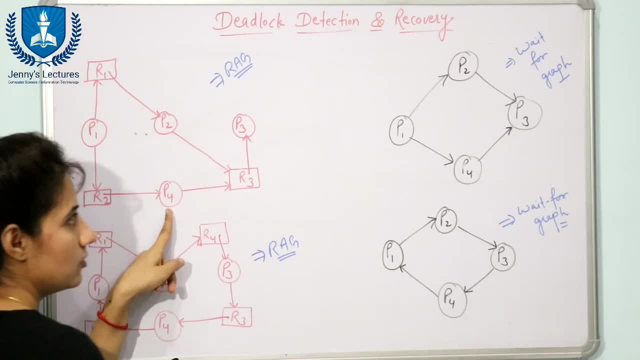 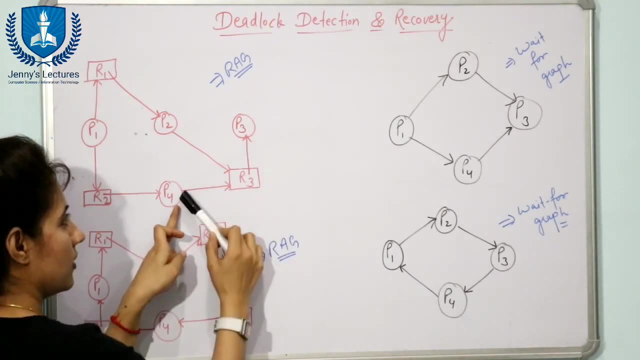 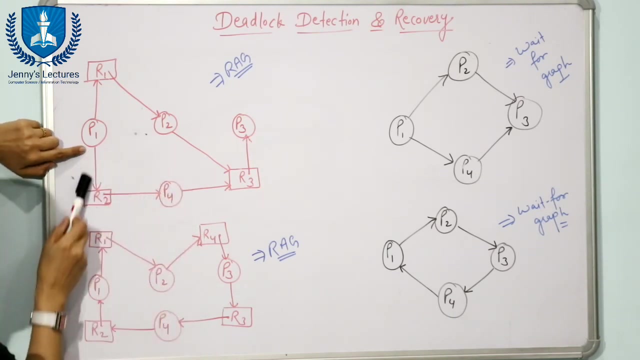 release this r3, so p4 is waiting for p3. remove this resource and this edge, this one, this one. just make one edge, like, like this: from p4 to p3, same with this type of: remove this p2, this edge is from this one, this one. so just put one edge from p1 to p4, p1 to 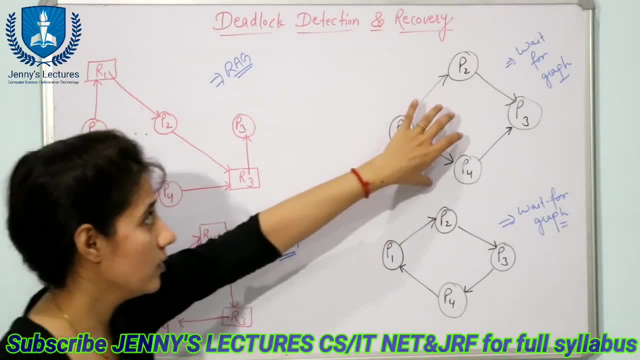 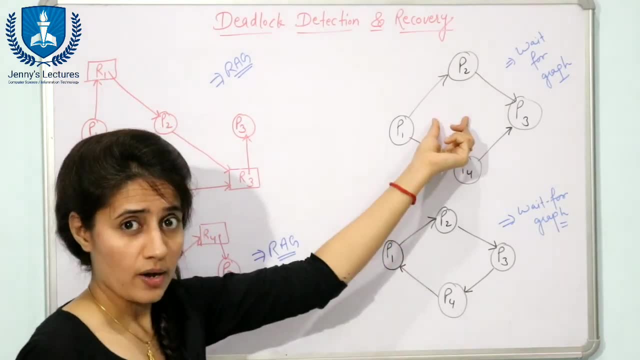 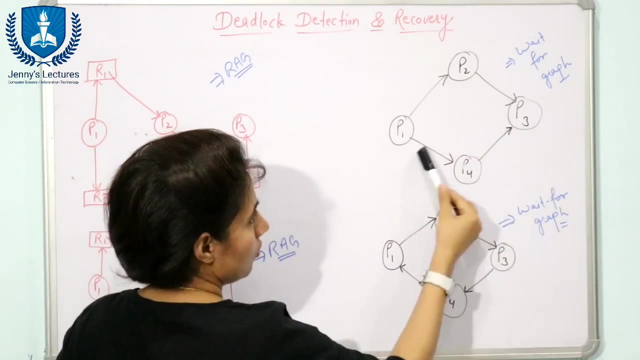 p2, p4. this is how we will construct a wait for graph from resource allocation graph. now, when the algorithm would be called on this wait for graph, then check whether cycle exists in this graph. see this one, this one, but this is not like this. this one, this one, but here is no outgoing edge. so there is no cycle in this wait for graph. so we can. 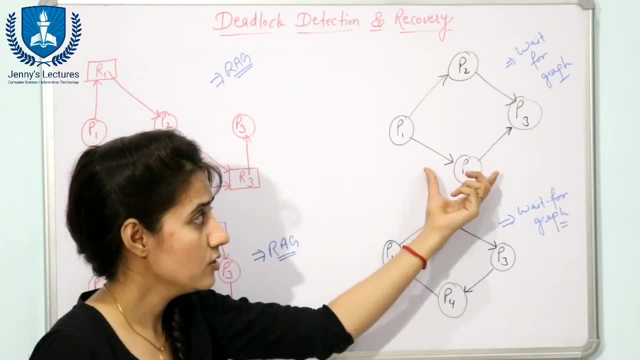 see at this particular state in the system. there is no deadlock because there is no cycle in this. involved in this cycle: because this девelope is an layered event. so when the algorithm does not wait for the systems, there is no dead look because there is no cycle in this gray area. so you get an. 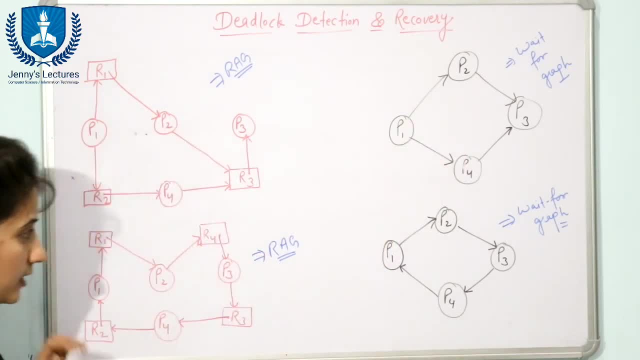 weight for graph. now let us take this example. this is another resource allocation graph and this is corresponding weight for graph for this one. simply how to construct: simply remove that resource edges from p1 to resource and from resource to p2. so simply put an edge from p1. 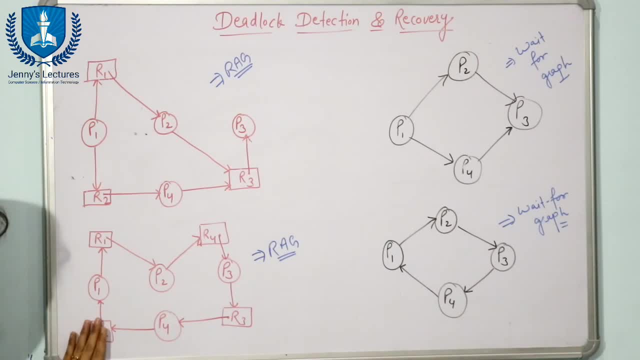 to p2, p1 to p2, like this: remove this. r2 edges from p4 to this resource and this resource to p1. so simply put an edge from p4 to p1, p4 to p1, like this: remove this one. from p2 to p3- remove this. 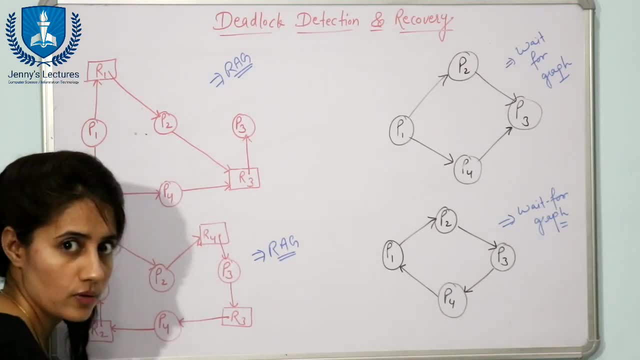 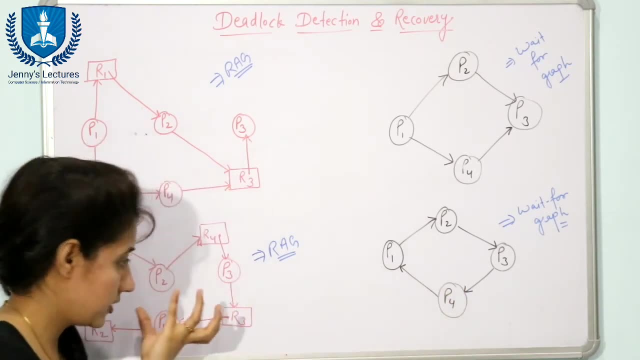 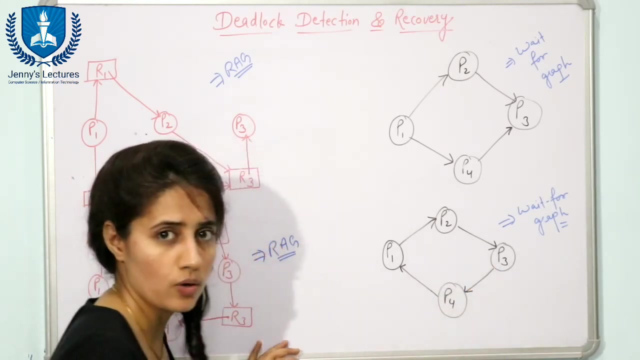 resource from p3 to p4, p3 to p4. now the algorithm system will call an algorithm on this weight for graph at this particular state, at this particular state of the system. fine, now check if there is cycle in this graph. yes, this one, this one, this one and this one. cycle means a closed loop, starting from one point and come to that point only. so, yes, it contains a cycle. it means there is deadlock. in this case, here, there is no deadlock. so now the main question is how frequently this deadlock detection algorithm would be called so this? this answer depends on mainly two factors. first, first thing is: 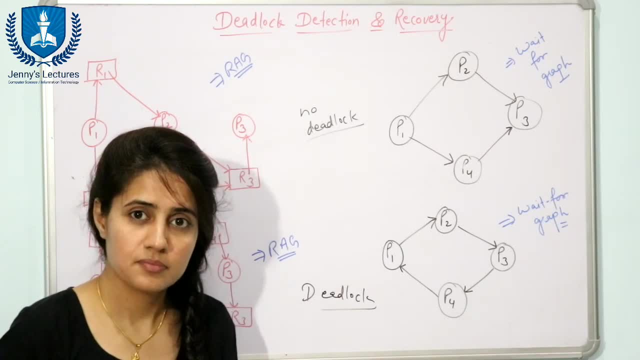 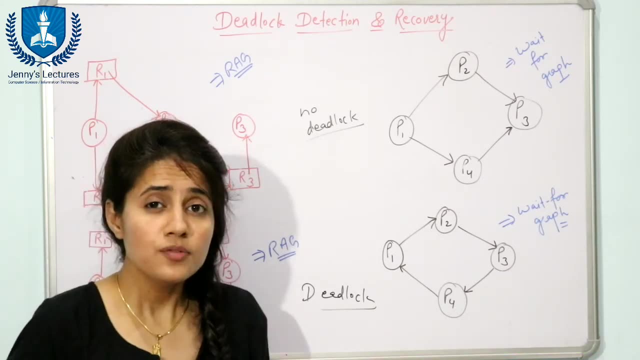 how frequently deadlock occur in the system, fine, and second point is how many processes will be affected from that deadlock. so if deadlock occur very frequently in the system, so obviously that detection algorithm would be called very frequently, fine, and second second thing is what see when a deadlock comes, when a system, when a process request some resource and 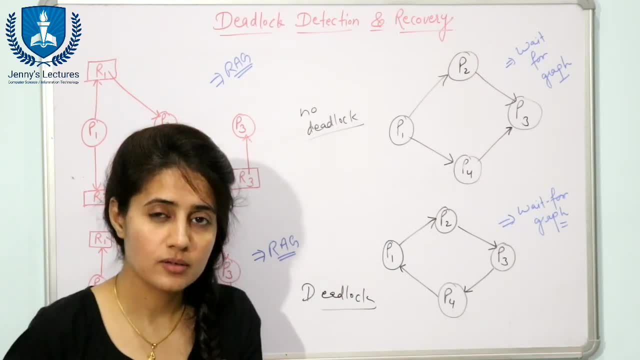 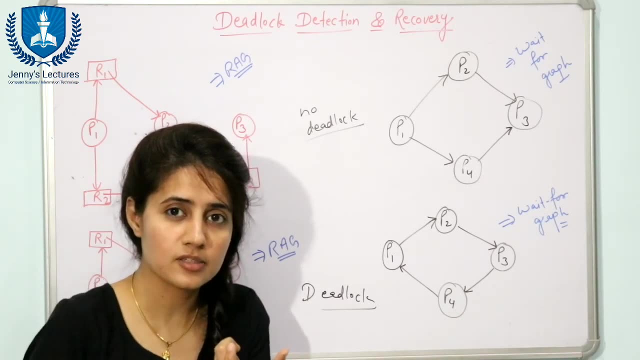 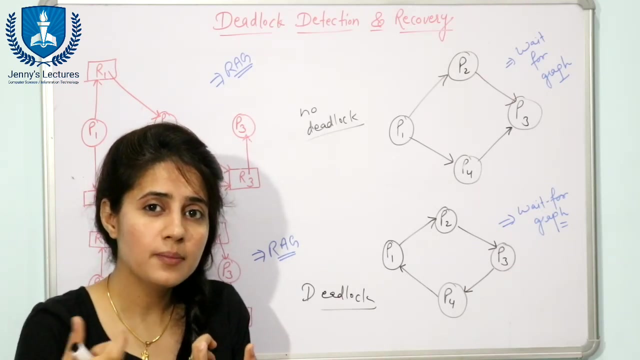 that resource cannot be granted immediately. fine, maybe those resources are held by some another process which is also in waiting state, something like this. so we can say that when a process request for some resource and that request cannot be granted immediately, if such case is there, then call detection algorithm. 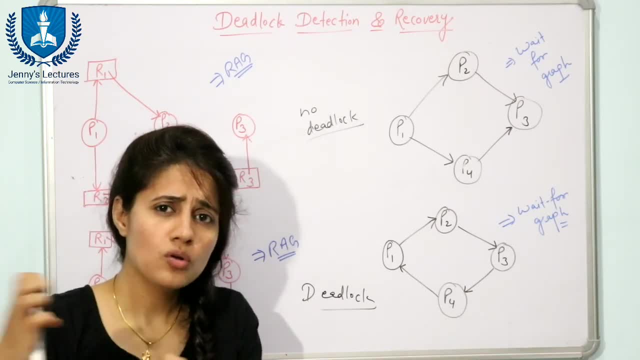 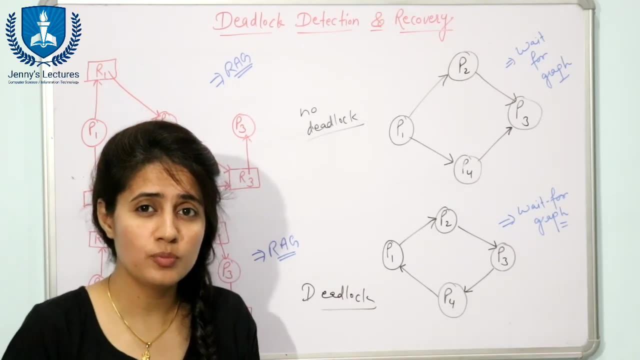 but if for every resource request we call the detection algorithm, then obviously there would be more overhead and obviously that computation time would be very high. so another alternative to this approach is: rather than calling the detection algorithm, for every resource request that cannot be granted immediately, just call, just invoke the algorithm after a defined interval, after a short. 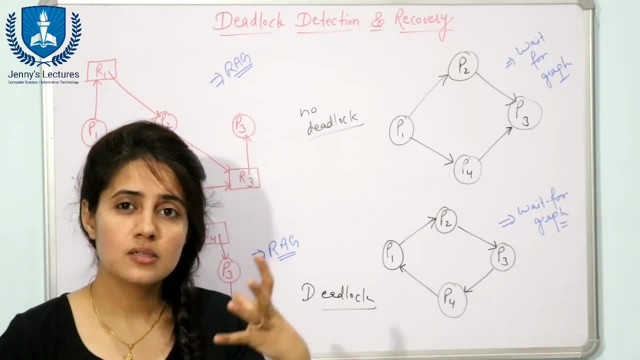 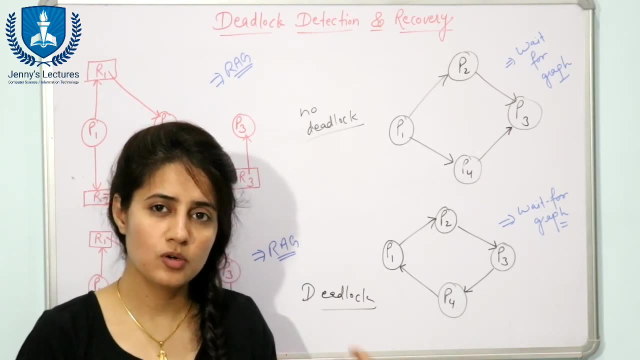 amount of time can, say once per hour, invoke the deadlock detection algorithm when cpu utilization drops below 30 or 40, something like this. see, obviously when deadlock will come, then it will affect the throughput of the system and obviously that it drops the cpu utilization. so if cpu utilization drops below 40, then uh, call the. 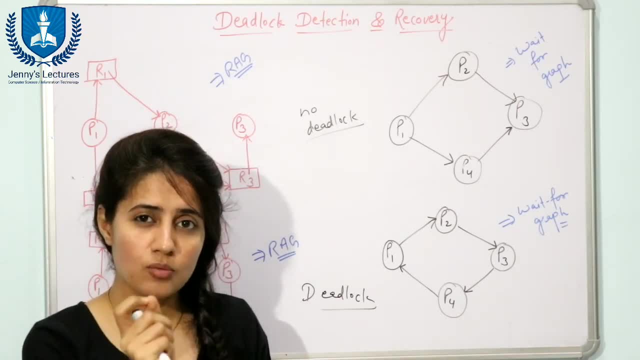 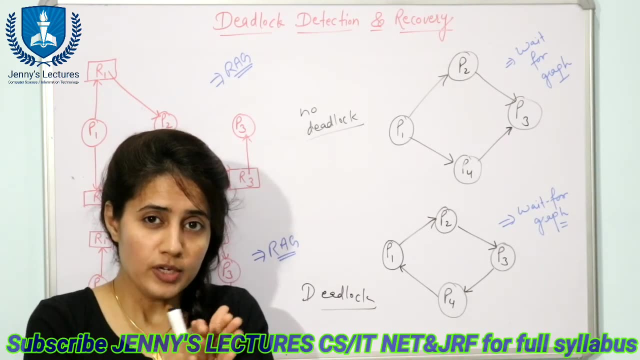 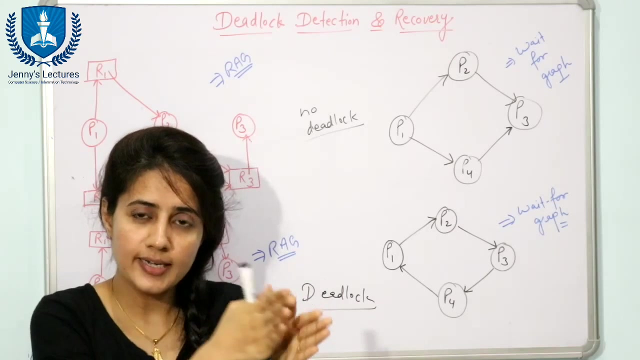 that detection algorithm. but you can that. the drawback of this thing is what if you call a detection algorithm after a defined interval, see during that interval of time? suppose you are calling that deadlock once per hour, so maybe during that hour at 10 o'clock that detection algorithm has been called and after that it will. 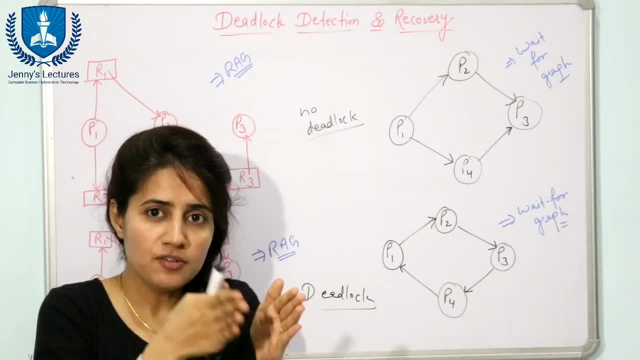 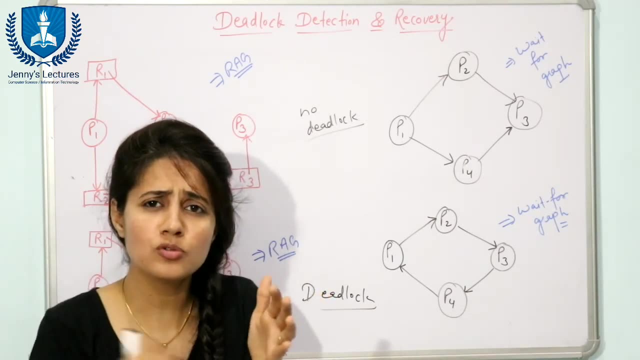 be called at 11 o'clock. so if at 10, 5, some some you know process got in deadlocked state, so till 11 o'clock more and more processes will be going into deadlocked state and when at 11 that that 11 o'clock when detection algorithm would be called, then many processes would be there in deadlocked. 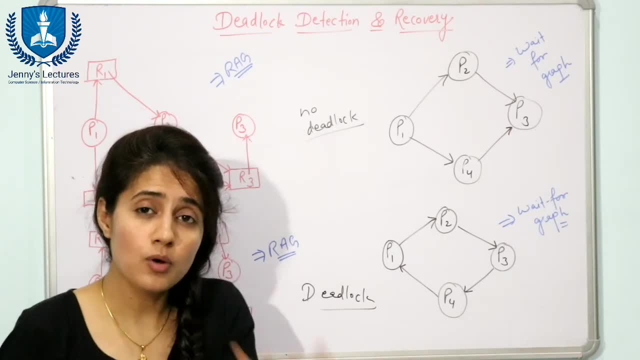 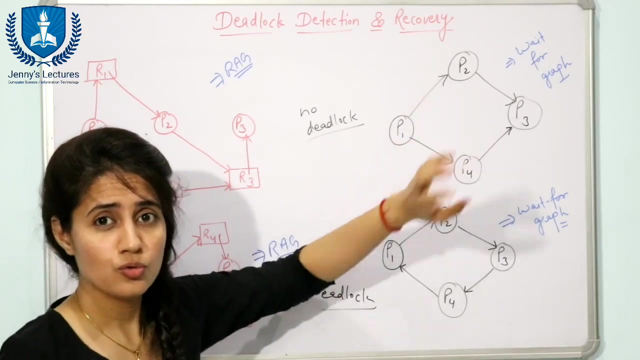 so at that time it would be, you know, impossible to find out that due to which process deadlock has arrived, or you can say which process is the main reason for this deadlock. so see, every every approach is having its own advantages and drawbacks. so this is how that wait for graph can be used to detect deadlock. now we will discuss. 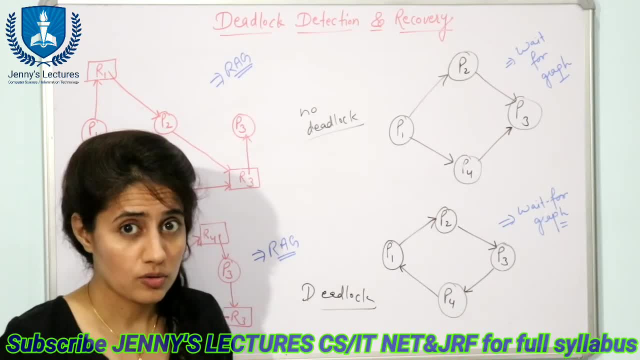 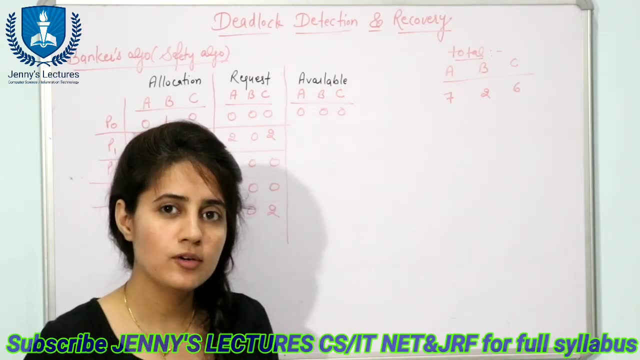 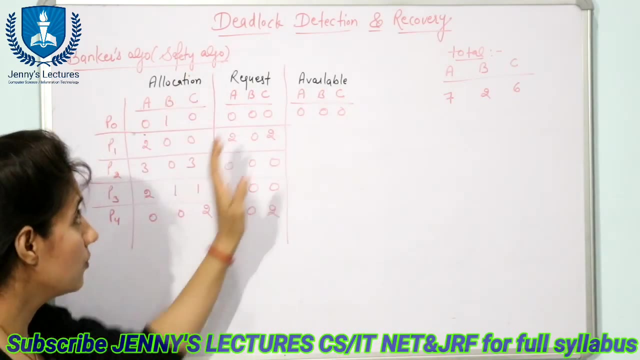 how benker's algorithm can be used to detect deadlock. so when multiple instances of resource resources are there, then benker's algorithm- or you can say safety algorithm- would be applied to detect deadlock. see, this is one snapshot. we are having five processes. allocation matrix is given request. 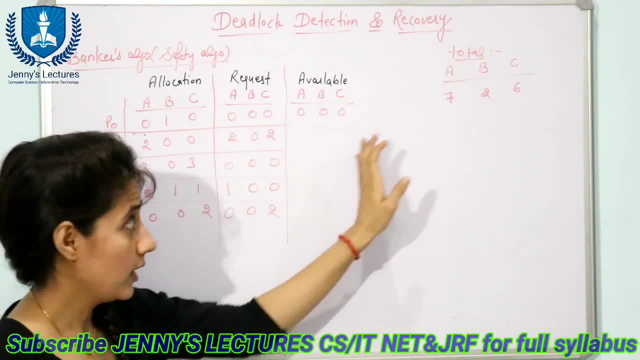 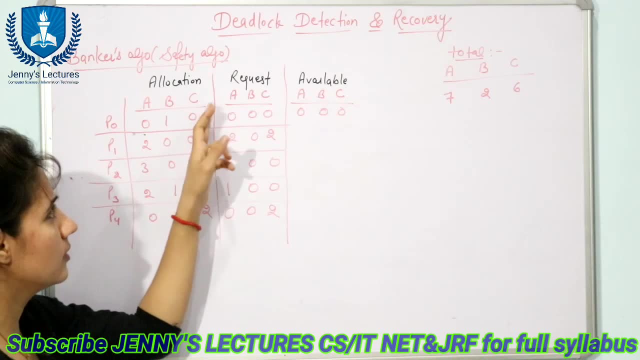 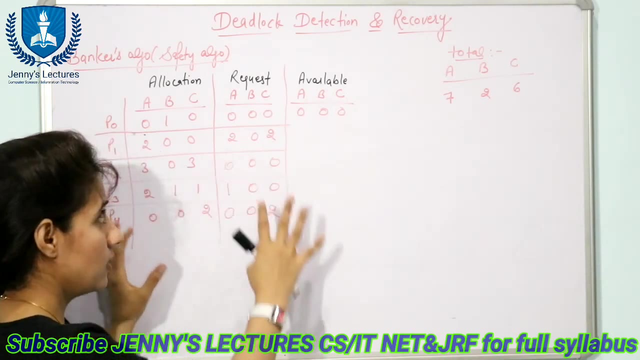 matrix is given and here available resources are given and these are total resources: a, b, c. a, b c are resource type. you have three resource type. maybe you can consider a, c, p, u, b's printer, c scanner, something like this. we have discussed benker's algorithm or safety algorithm in previous video, so i'm not going to apply that algorithm. 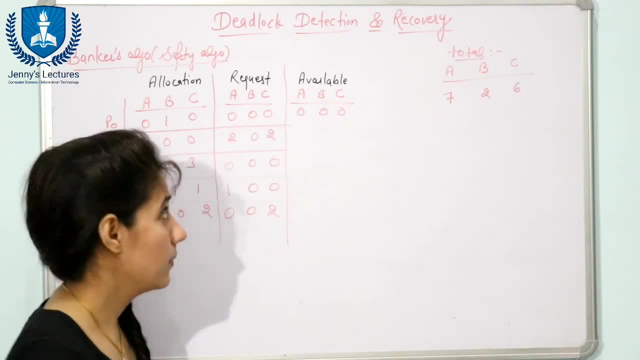 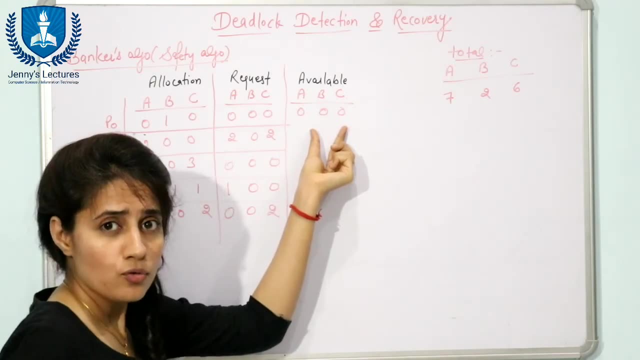 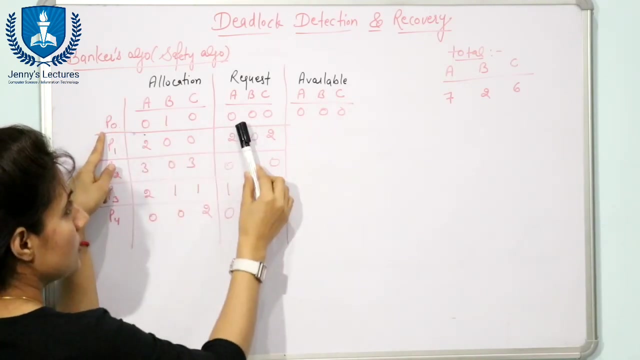 properly here you can check out in previous video i'll provide you the link. see here. this is the request matrix and zero zero, zero are available resources we have. so you have to check it out- which request you can fulfill with these available resources. see for p2 request is zero zero, zero. fine, it is also zero zero, zero. so you can take either p note or 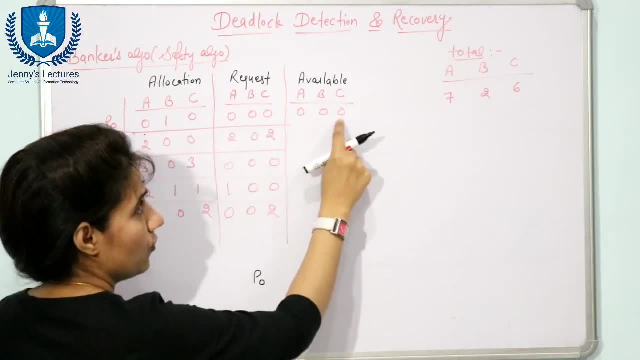 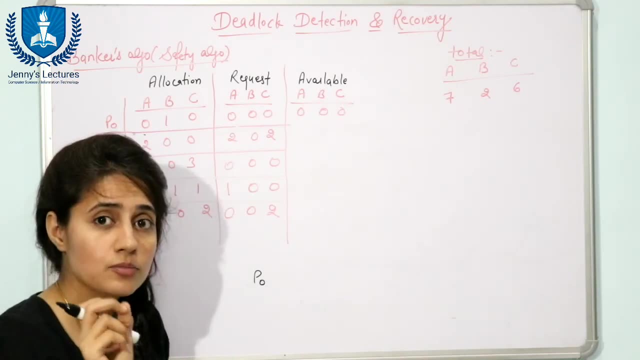 p2, so i am taking p note. i can fulfill this request with these available resources because this requi, this process, does not need any resource. the assumption is, when we apply benker's algorithm, as soon as a process gets all its required resources and then it will release its resources, fine, maybe. 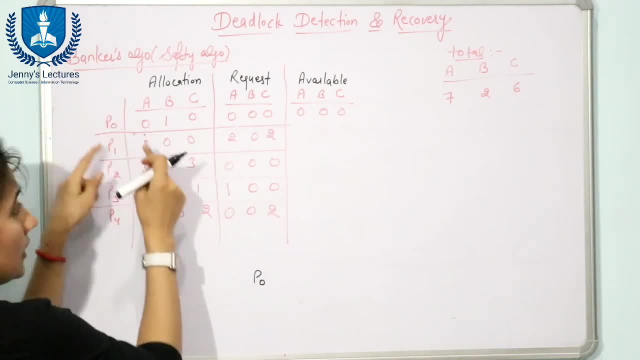 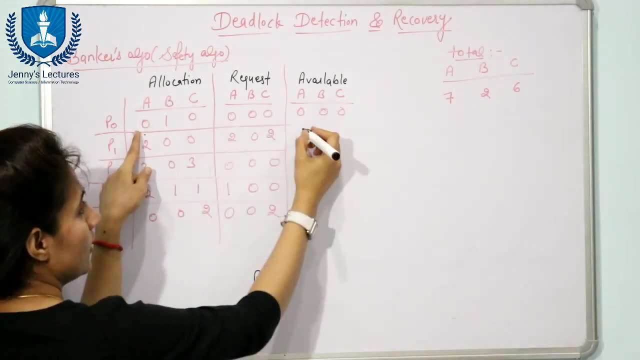 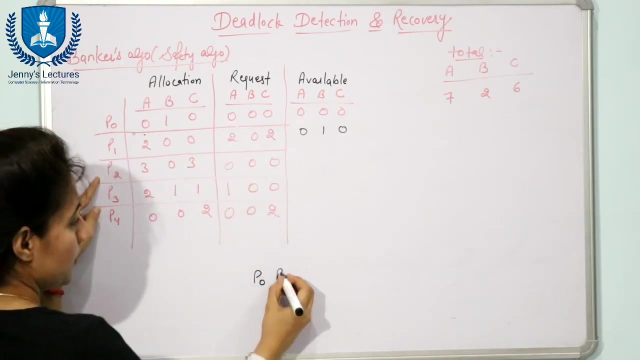 some finite amount of time. so this process will release its, its resources and what we will do? in available we will add a location. allocated resources: zero one, zero. so now available resources are zero one, zero. now, with these available resources you can fulfill which request, i guess p2 request. it also needs zero, zero, zero. so as soon as it gets, uh, as soon as p2 got completed, it will. 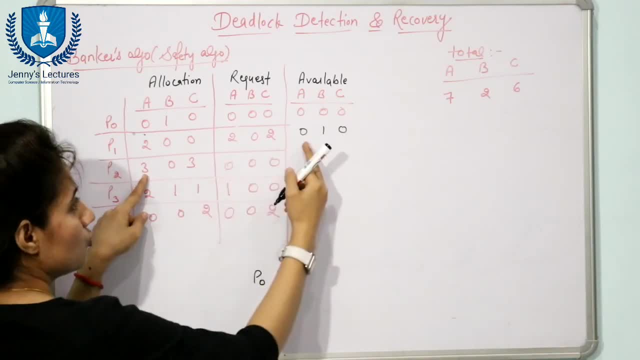 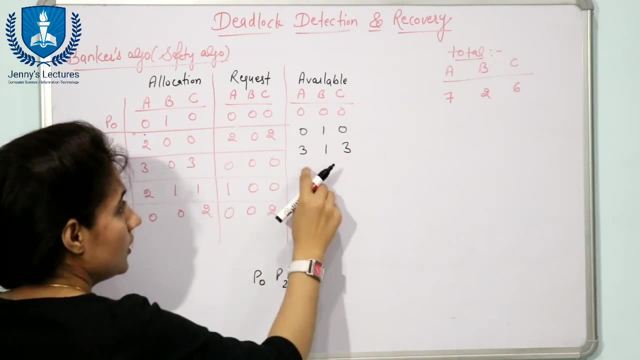 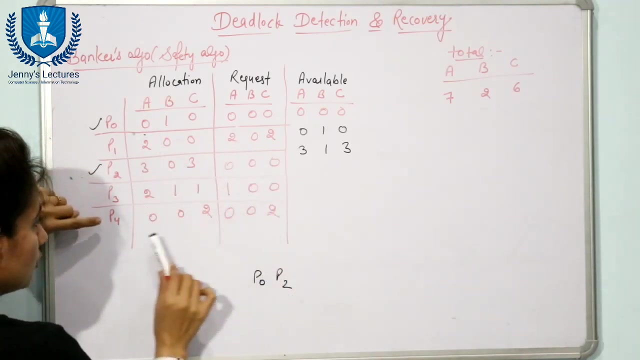 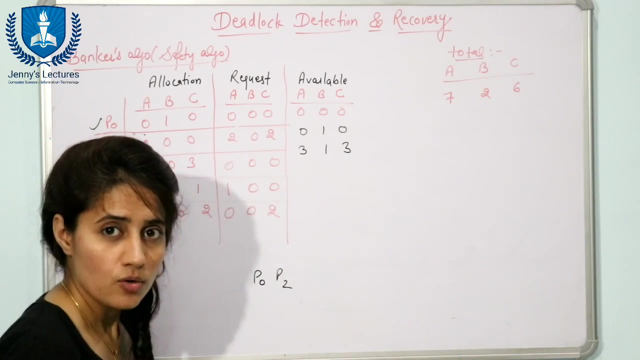 release all its resources now. add these allocated resources to available resources, now available sources would we would become three. one and three now with these available resources. see these two got completed. now you can fulfill this request also. you can fulfill this request also and you can fulfill this request also. fine, so ultimately, when you will apply that bankers algorithm? 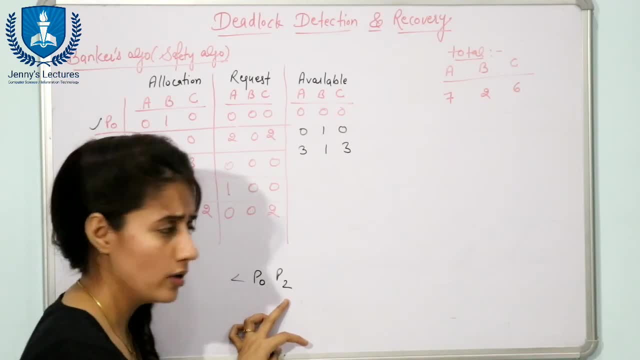 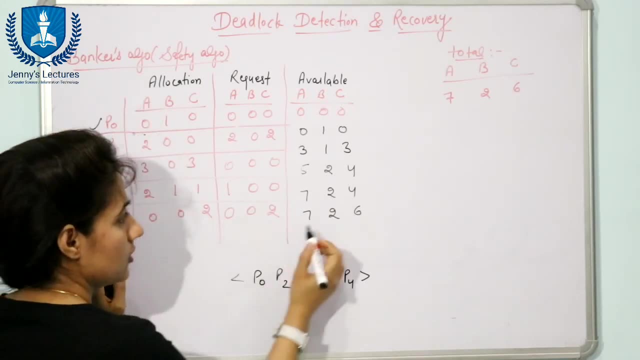 then you will find a safe sequence, and that safe sequence would be: what now, when you will apply the banker's algorithm? ultimately, you will find this safe sequence fine and after, excuse me, executing all the processes. these are the available resources: 7 to 6 and total resources. 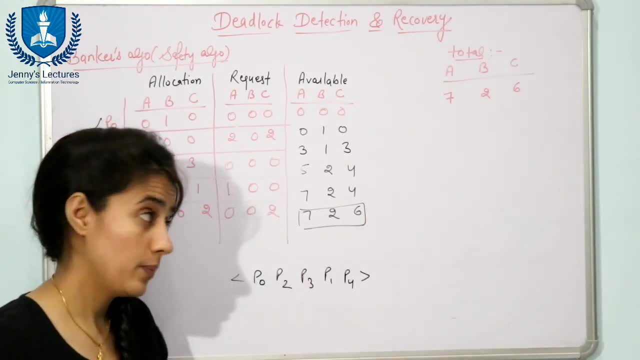 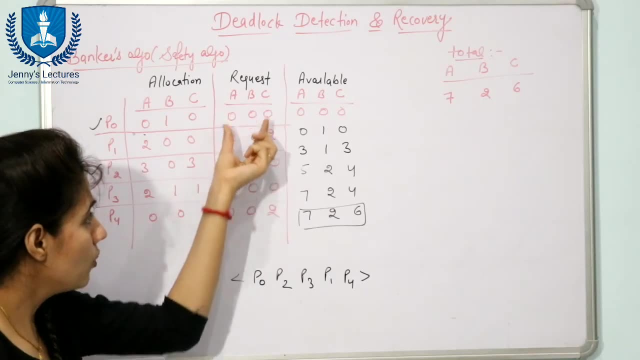 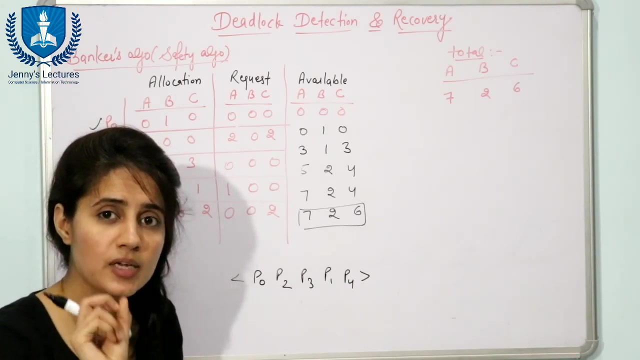 are 7 to 6, so we are going at right path. fine, so here you can say there is no deadlock because you are able to- you are able to, you know- fulfill all the request without going into unsafe state. so there is no deadlock. now, if the situation is something like this- see, if this request 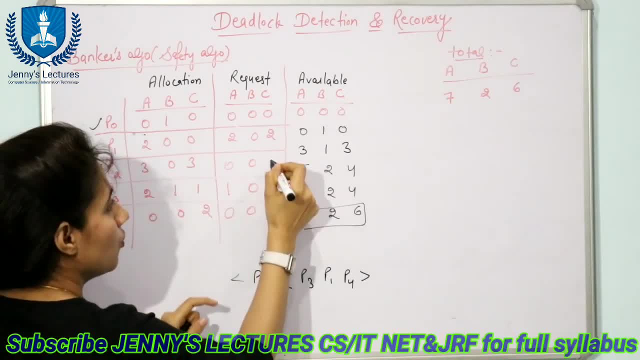 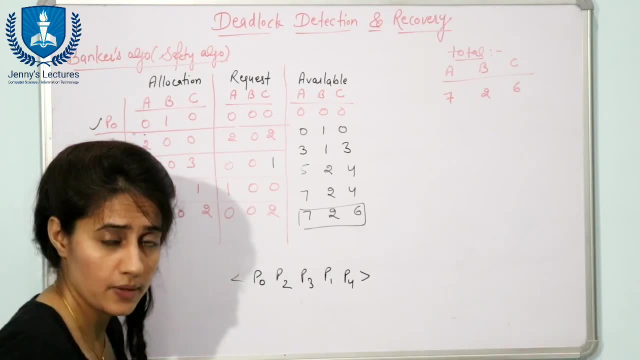 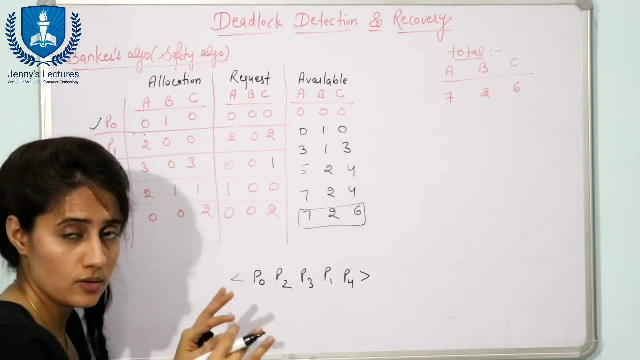 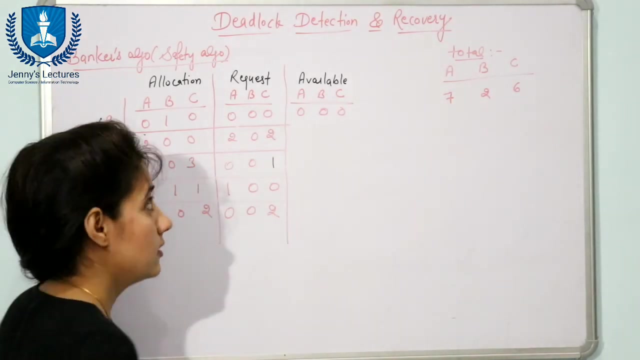 of this P2 is 001. see this snapshot is there at some at particular time in the system. now what will happen? available resources are 000. now you have to find out. this system is in safe state or in deadlocked state. so now again, apply safety algorithm, or you can say bankers. 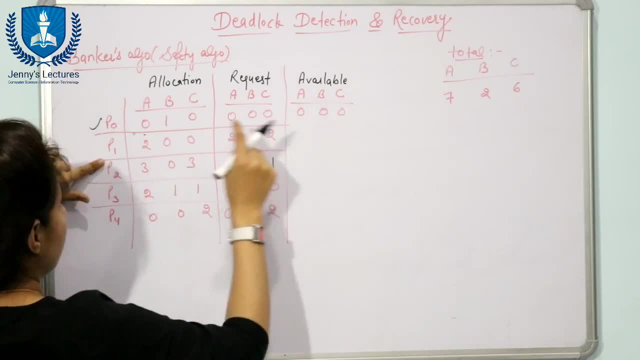 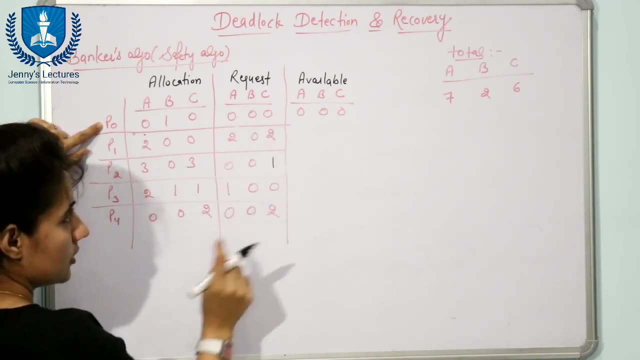 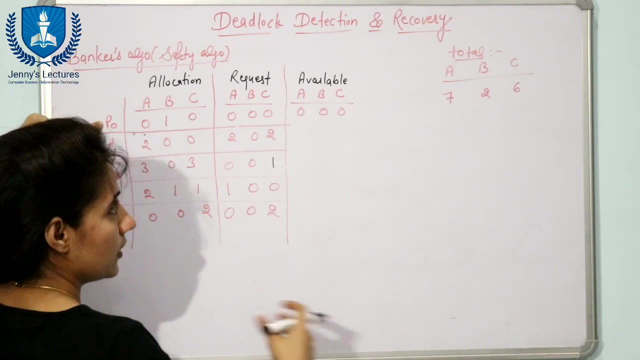 algorithm. see, with these available resources I guess you can fulfill request of only P2 000.. So these two addresses are there in регulatory state. Yeah, fine, we cannot fulfill this request. not this, not this and not this. So when not gets all its resources, it will release all its. it will you know. finished. 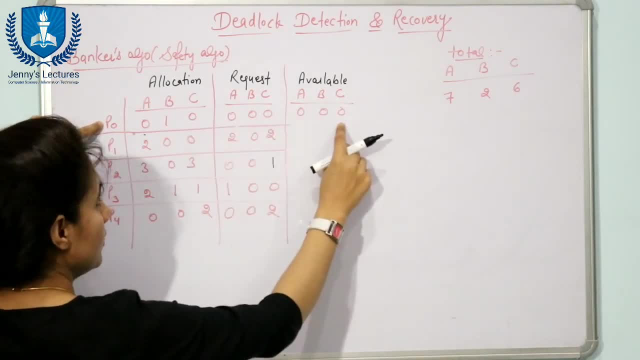 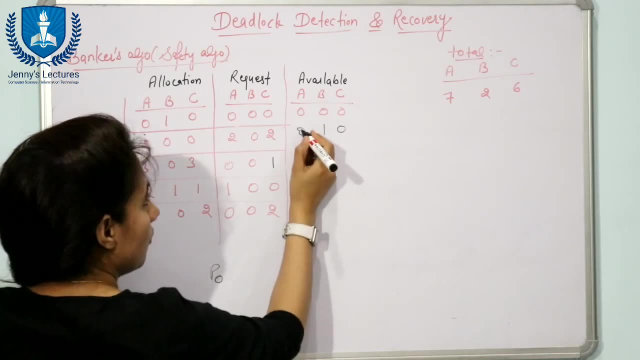 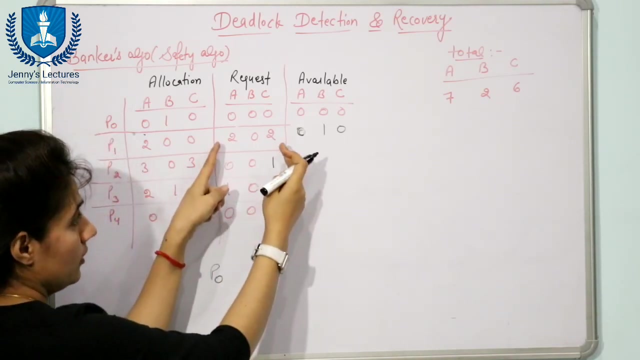 its execution and it will release all its resources. So now in availability sources we add allocation resources of P0- 010. now available resources are 010 and P0 got completed Now. you can now look at the pages. By the way, did you see the outdoor dayục anyways? 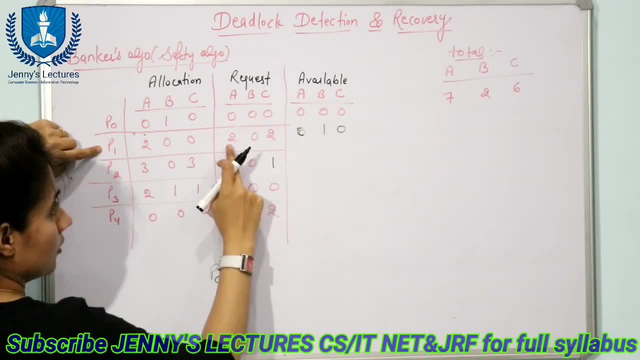 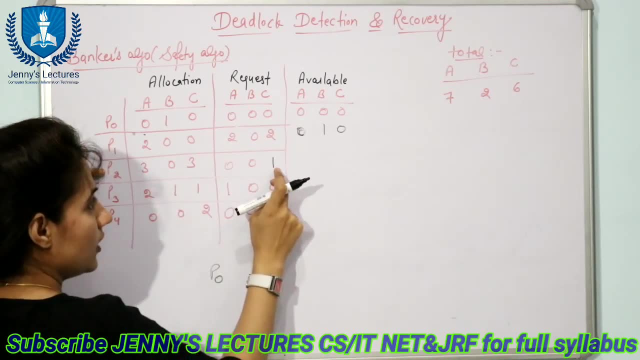 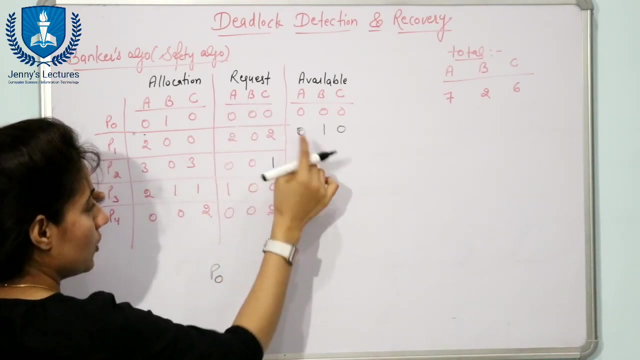 Now check which request you can fulfill. P1, 2: it required 2 instance of A, but we have 0. we cannot fulfill this request. P2: it require 1 instance of C, but we have 0, so you cannot fulfill this request. P3: it require 1 instance of A, but we have 0. it requires 2 instance. 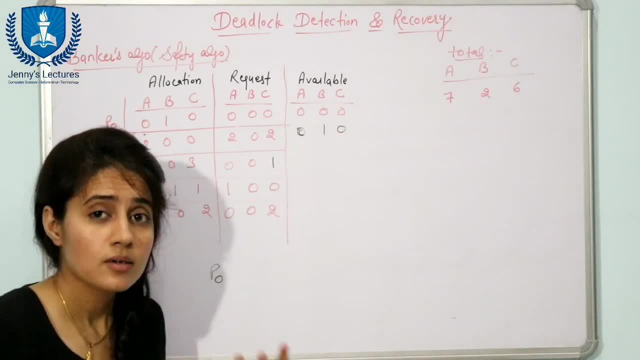 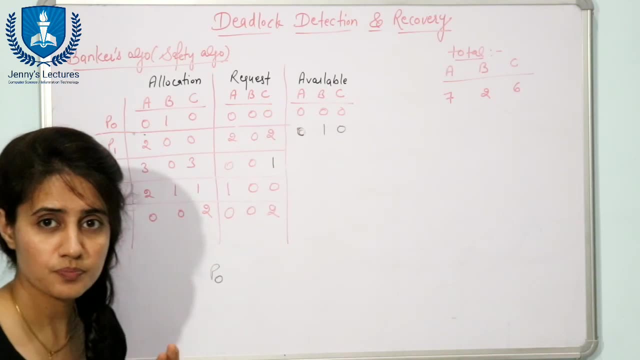 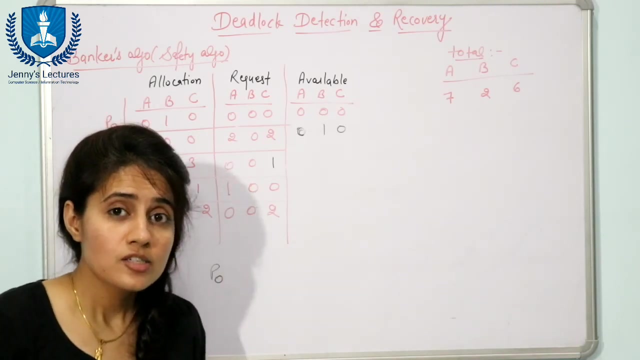 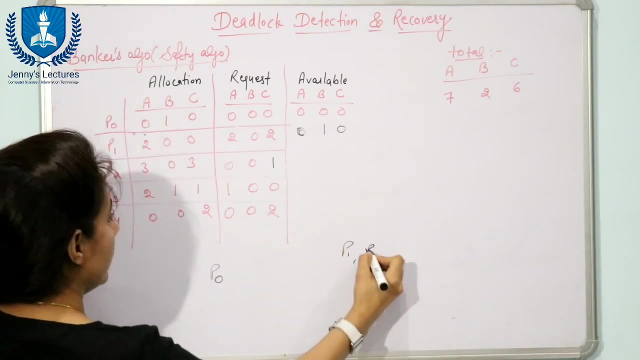 of C but we have 0. Now system is in a state in which it cannot fulfill request of any of the process, any of the remaining process. now we can say system is in deadlocked state. and if you are asked which processes are in deadlocked state, so P1, P2, P3 and P4, these 4 processes except. 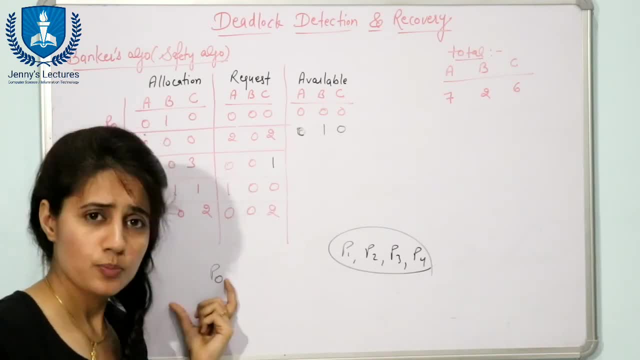 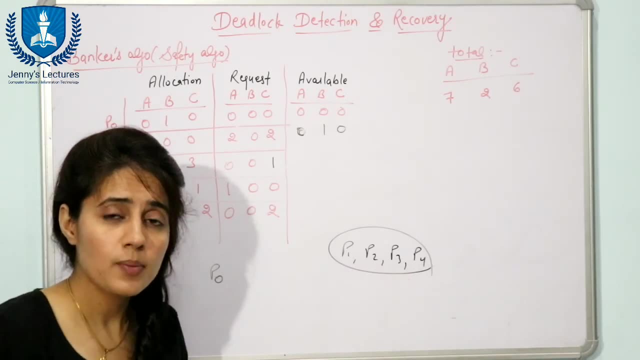 P0,. P0 is not in deadlocked state because P0 got completed. these processes are in deadlocked state. So this is how you will apply bankers algorithm, or you can say safety algorithm to check system is in deadlocked state or not. here I am taking request matrix in that case, in deadlock avoidance, 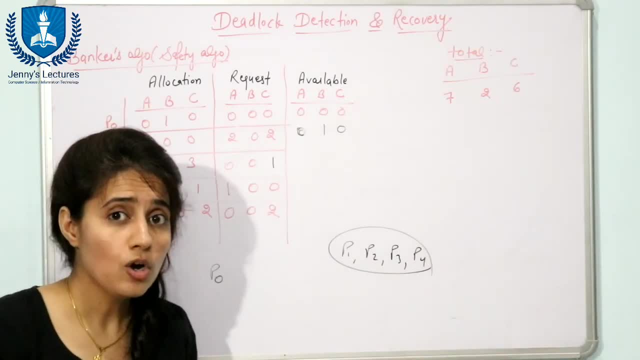 we have taken need matrix and all so because deadlock. deadlock will come when system is not able to fulfill any request immediately. fine, then obviously deadlock will come. so here, that is why I am taking request matrix of P2.. See, the steps are same. we have same, as we have discussed in safety algorithm, when we 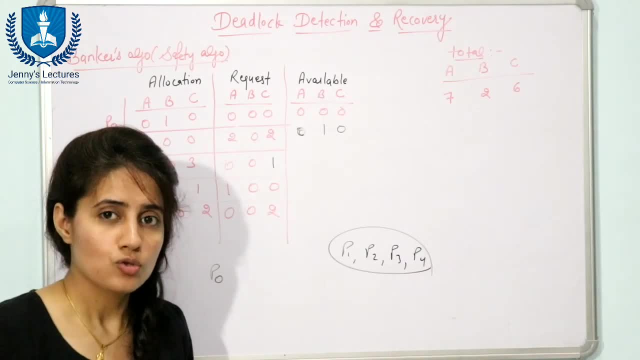 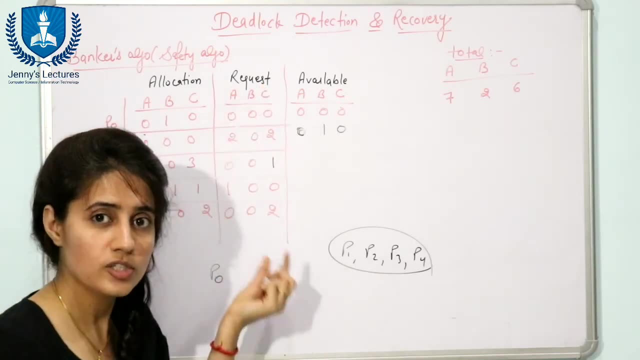 were discussing bankers algorithm in deadlock avoidance, so just check out that video. in that algorithm we have taken need matrix, but here you will write what request you will check. request is less than equal to available, then fulfill that request. otherwise you will set one flag variable. 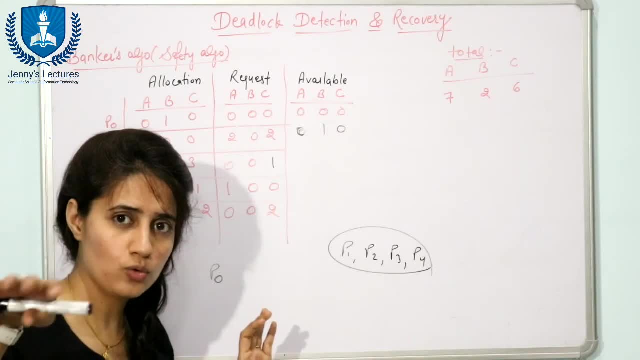 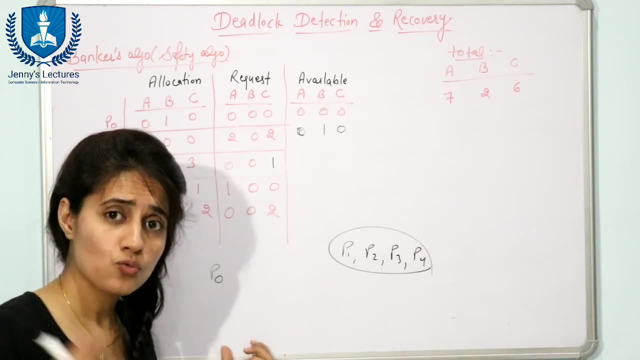 If you find any flag variable of any process is equal to 0 or you can say false, then you can say system is in deadlocked state. and if flag variable of all the processes is one or you can say true, then you can say deadlock is not there in the system. 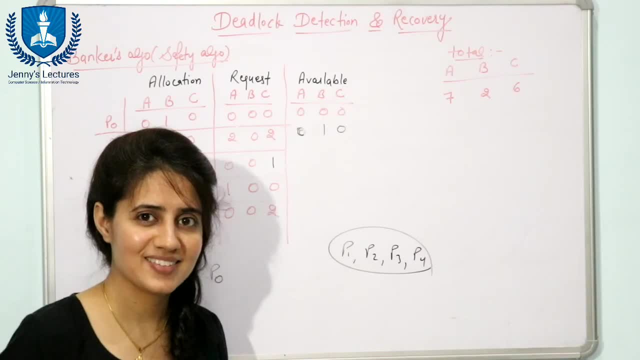 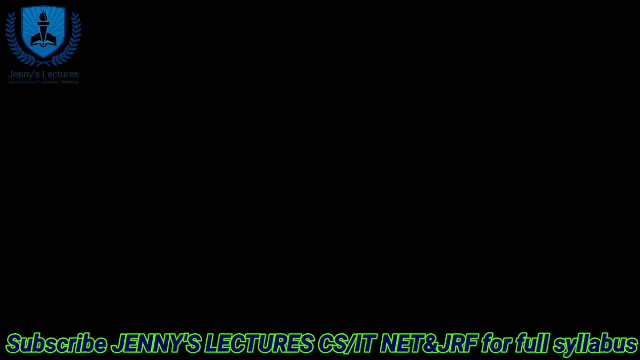 In next video we will discuss some recovery techniques. till then, bye, bye, take care.